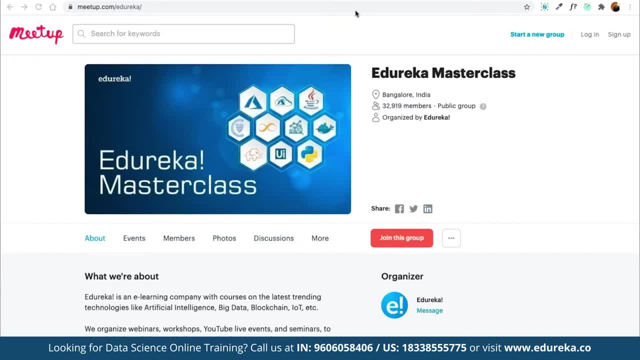 been closing into more than 32,000 members so far, and in these masterclasses we have been conducting multiple webinars and live events on different topics, including blockchain, IoT, artificial intelligence, machine learning, big data and multiple front-end and back-end development technologies. 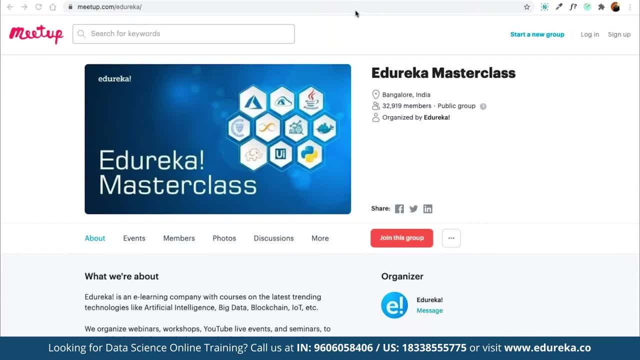 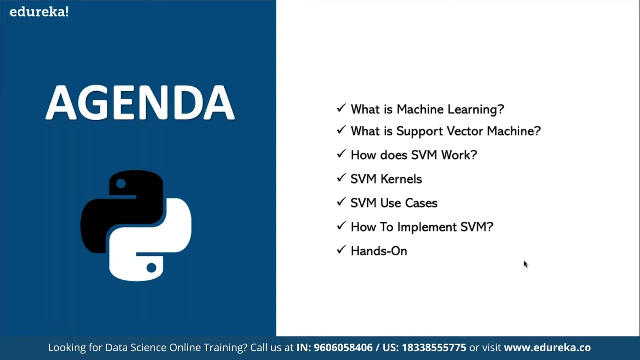 So here we are going to start our discussion on SVM, as in support vector machine, How exactly this is structured and how exactly this is going to be helpful for us. So first of all, we are going to talk about what exactly is machine learning- to have a quick clarity on that, and then we are going 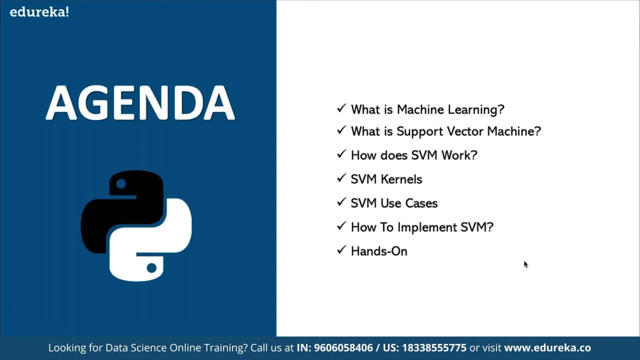 to talk about what exactly is support vector machine, and then we'll talk about how exactly it works, and then we'll talk about the SVM kernels and then we are going to talk about the components of that process of implementation of SVM as a part of a discussion and if time allows and we can also see a small hands-on. 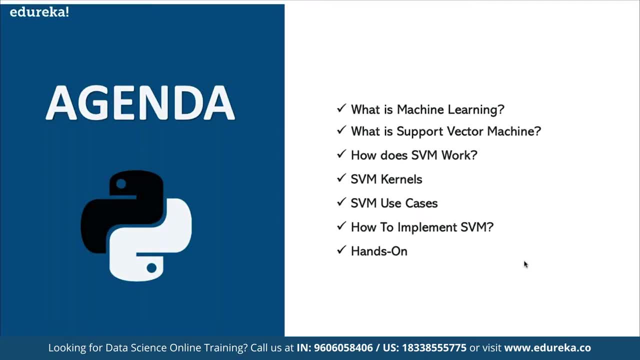 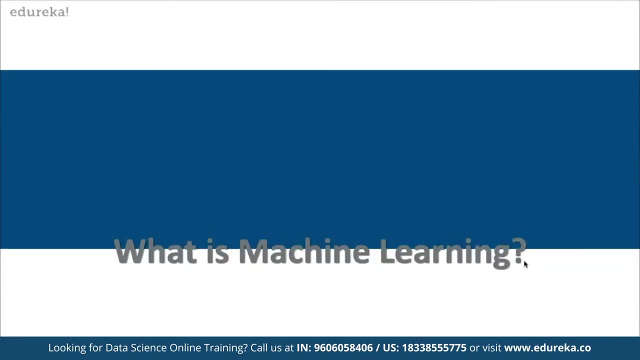 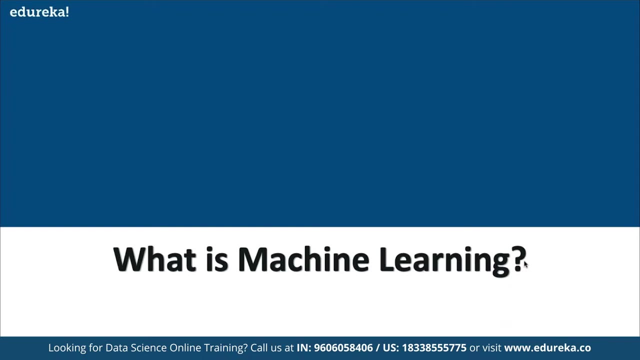 on top of it as well. All right, so first of all, if we talk about machine learning itself, so what exactly is machine learning? So machine learning is simply making sure that we are going to automate the system by using a good amount of data set right, So we can say: machine learning is simply. 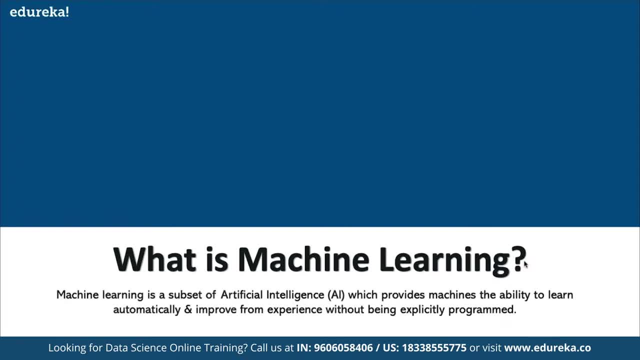 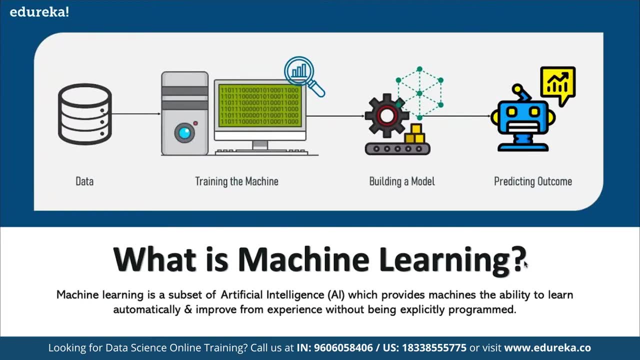 the process of feeding a machine enough data to train and predict a possible outcome using the algorithms which we have the access to. So, basically, if we use more data set, then we can increase the accuracy of the results and, let's say, you may have used multiple predictions. 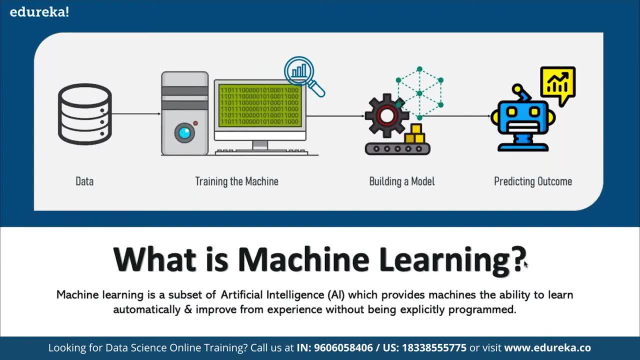 made in support before any major match right. So in this case let's take an example for a football penalty session. So the data of previous performances are going to be considered. So let's say the goalkeeper has saved all the penalties to his right in the last 50 penalties he has saved. Now this data will 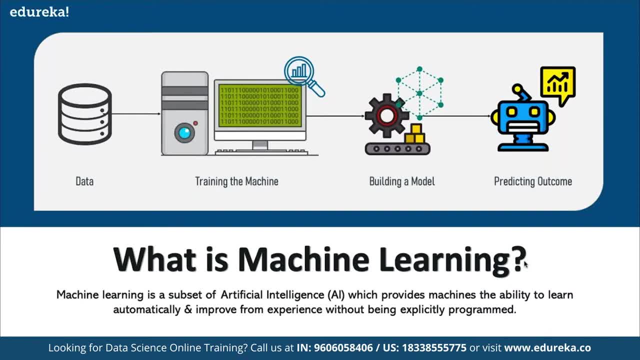 be crucial to predicting if he or will will save, or he will not save, the next penalty phases. So there are other factors to consider as well, and another example can be the suggestion that we get while surfing the internet. So the data of our previous choices are processed. 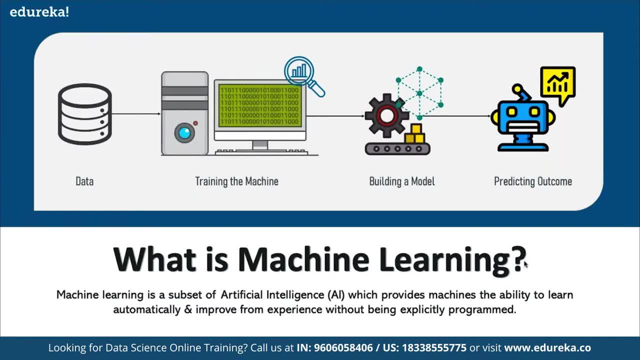 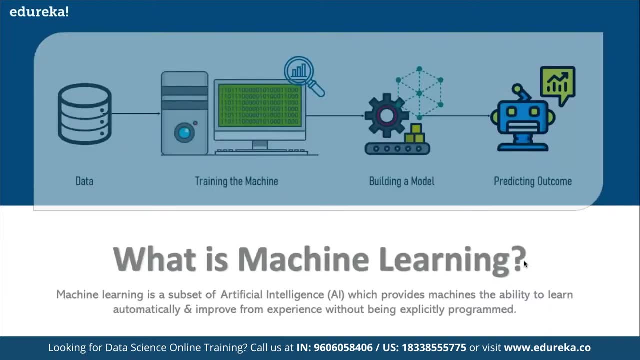 to give us the most favorable content we are most likely to watch. Anyhow, machine learning is just feeding the machine an ample amount of data. There goes a lot of processes, algorithms and decisive factors to get the optimum results. All right. so here, basically, we have three main types. 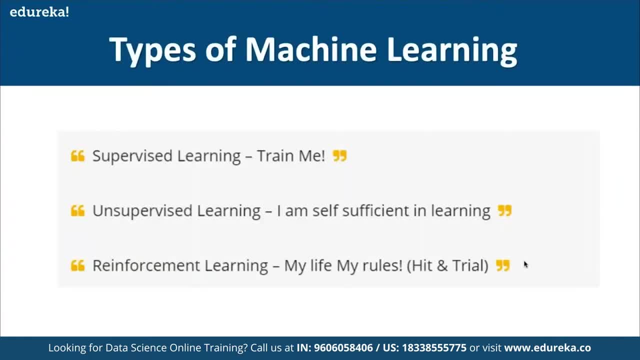 of machine learning as well, where we have supervised, unsupervised, and then we have reinforcement learning. So supervised in simple terms is: train me. It works on a simple training model. We have a training model, then only it can work, And an unsupervised learning is. 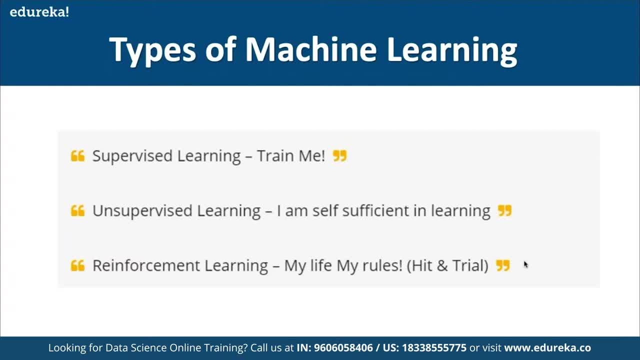 self-sufficient and learning based on their own learning. We are simply going to allow them to have, we're going to allow them to have the access as well. So that is what we are going to define. So, based on their own understanding, they are going to work accordingly. 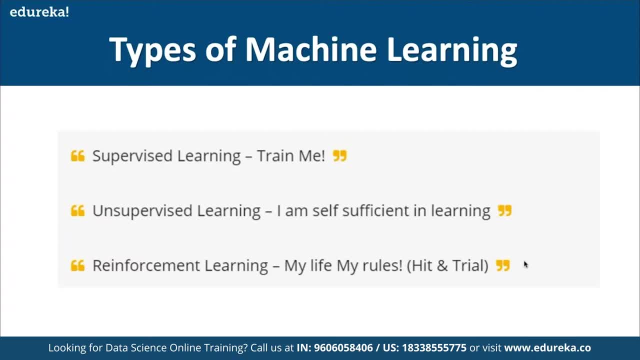 That's how it's going to work, And then we are going to work on reinforcement learning. So reinforcement learning is simply learning on its own, Based on the feedback. we simply train, we simply let the system know if they have done a good job, or 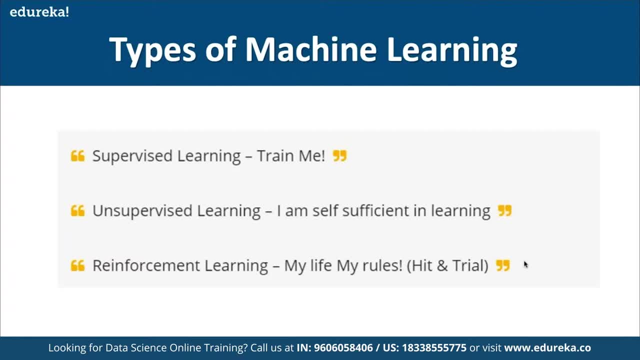 not, And based on that only, they simply try to get the best possible output. that's how it works, All right. So in supervised learning we use multiple labeled data set to train the system, And under unsupervised learning we use unlabeled data set, So the data is sometimes unlabeled. 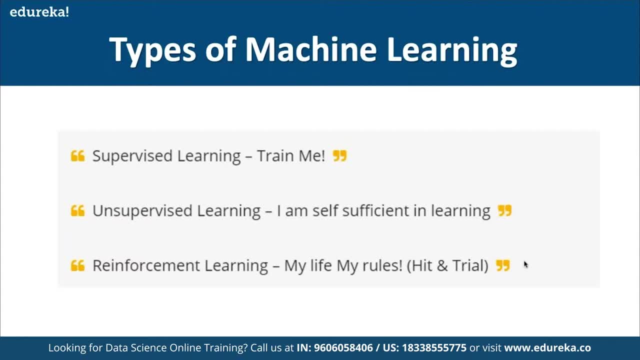 or we can say uncategorized, and the machine makes the best, the best possible reference. And then we have reinforcement learning. So reinforcement learning simply ensures that we are simply going to create a system based on the feedback. So the machine needs to establish a systematic pattern of approach in reinforcement learning. So that's. 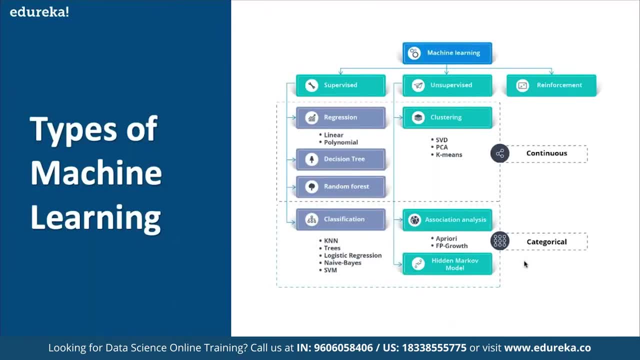 how we discuss Again here we have supervised, Again under supervised, we have multiple models Like we have regression decision tree, we have reinforcement models. we have different models currently available, Whereas in under unsupervised we have multiple models. We have clustering, we have association analysis. 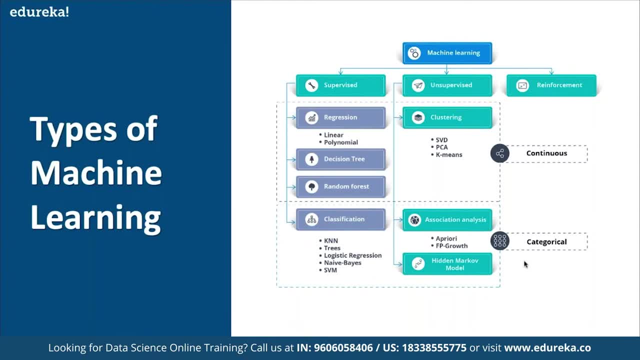 we have made in Markov model. So again, the KNN trees, logistics, regression and SVIM. they all have types of classification Where, if we talk about the upper theory, II grow. gay means PCA, SVD. they all are part of unsupervised. and again, 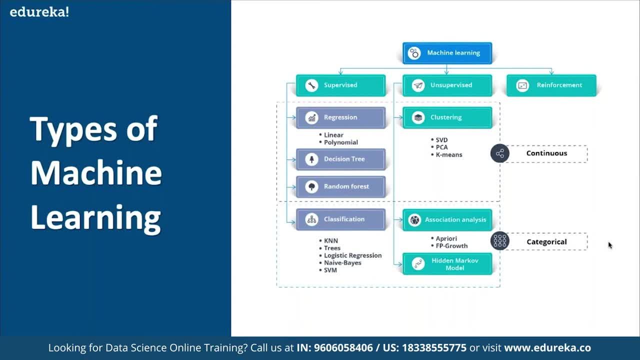 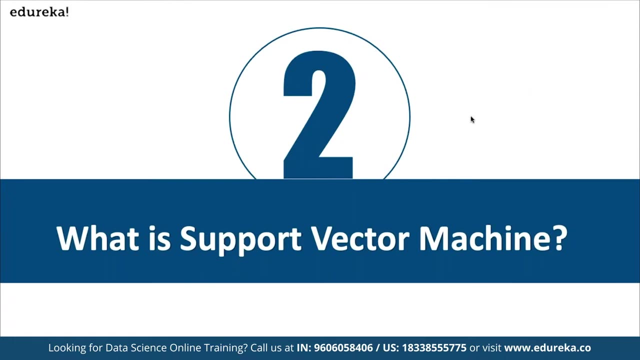 reinforcement is simply based on its own structure. that we are going to discuss as we proceed for the stepby step. all right, so now. next is we are going to discuss on what exactly we mean by support vector machine. so a support vector machine was first introduced in the 1960s and later. 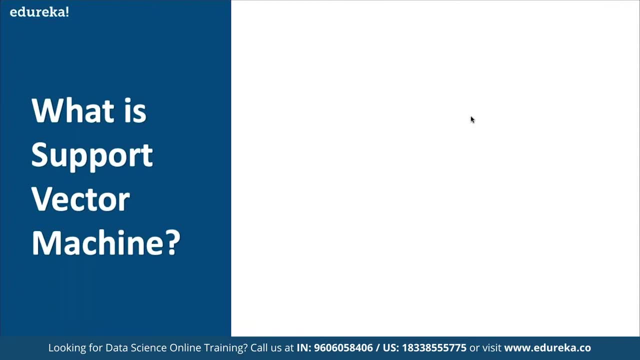 improvised in 1990s as well, and it is basically a supervised learning machine classification algorithm that has become extremely popular nowadays because of its- you can say- efficient results and especially for the complicated scenarios. it can deliver it for us as a part of support vector machine. as you can see again, it simply is like a discriminative classifier that. 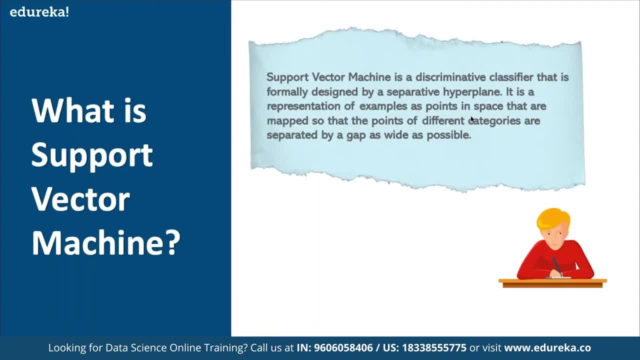 is formally designed by a separative hyperplane itself, and svm is implemented in a slightly different way than the other machine learning algorithms, so it is capable of performing classification, regression and outlier direction as well, and support vector machine is basically again simply designed by as a separative hyperplane instead, as we discussed. so basically, here we can have: 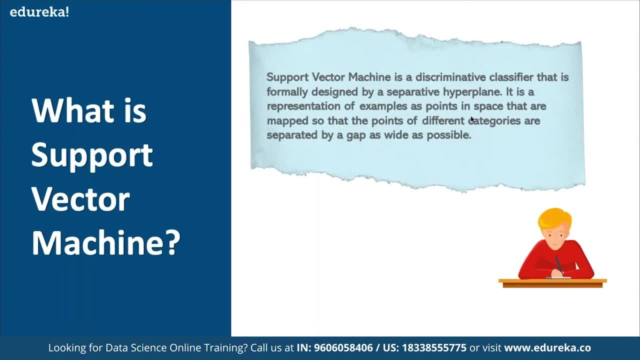 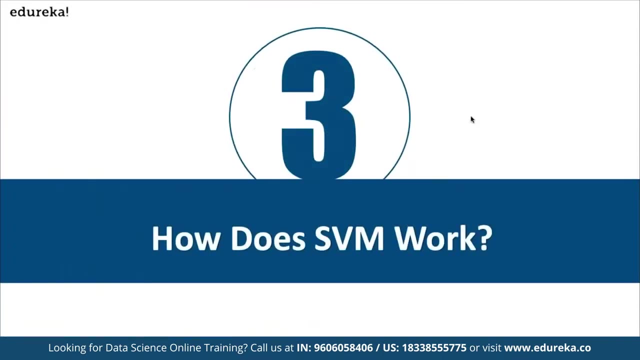 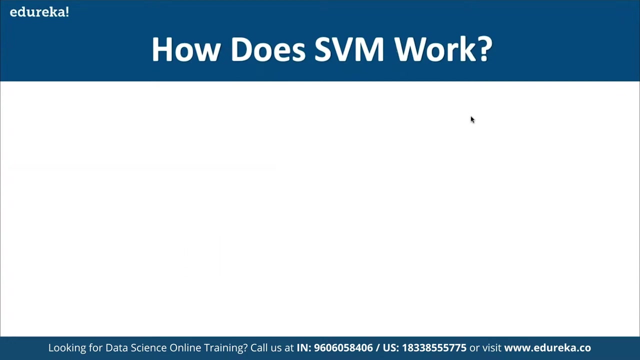 multiple data pointers that can be mapped, so that the points of different categories are going to be separated by a gap, and in addition, so basically, svm can also perform non-linear classification. so we'll be talking more about the how exactly support vector machine works as we proceed further. but there are multiple advantages of using svm as well. 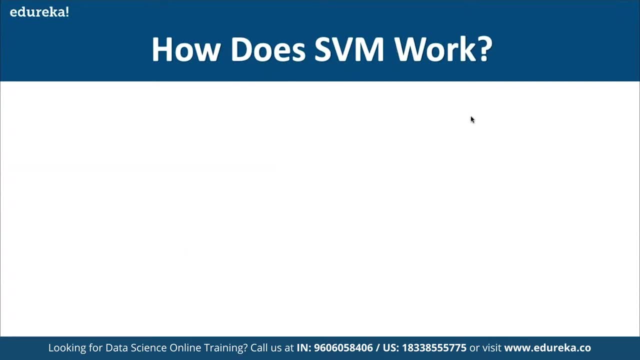 for example, it is effective in high dimensional spaces. it is effective in cases where the number of dimensions in greater is greater than the number of samples, and it is okay. it simply uses a subset of trading points in decision function. that makes it memory efficient and it has different kernel functions. 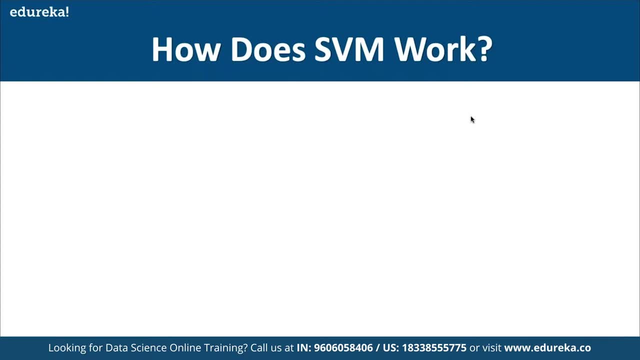 that can be specified for decision function. that also makes it versatile. and the same way we also have multiple, we can say downside or we can say disadvantages of using svm as well. so, for example, we can say that we have a number of features that are much larger than the number of samples. 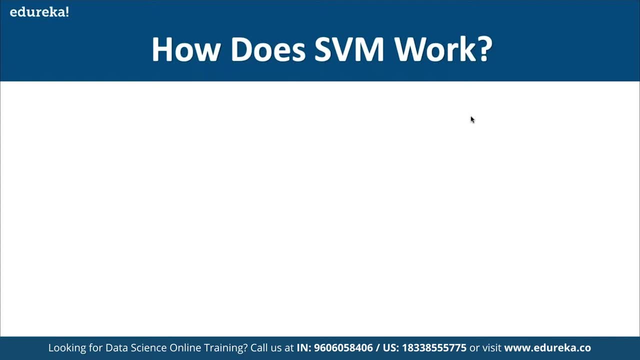 then we can simply avoid overfitting and choosing kernel functions. and again, recognizing them is crucial. and svm did not directly provide probability estimates and these are calculated using the five fold cross validation. and how does svm work? so the main objective of a support vector machine is to segregate their given data in the best possible way and when the segregation is done, 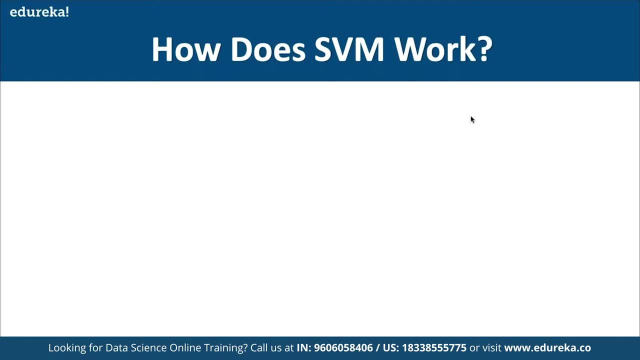 the distance between nearest point is known as the margin, and the approach is set to a hyper, basically hyper- plane with the maximum possible margin in the support vector, as we can see here. that has been right now presented all right and now basically here to select the maximum hyperplane. 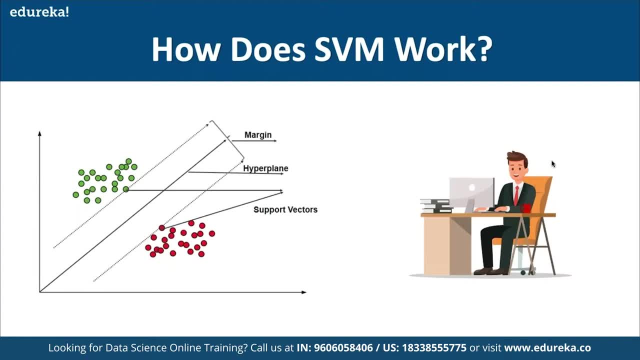 so now, in the given sets, the support vector machine follows again. multiple sets, for example- is simply going to generate the hyperplane which segregates the classic classes in the best possible way, and then we are going to select the right hyperplane with the maximum segregation from either nearest data pointers. so basically, 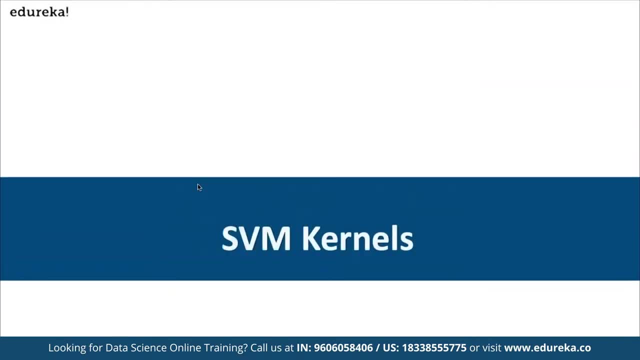 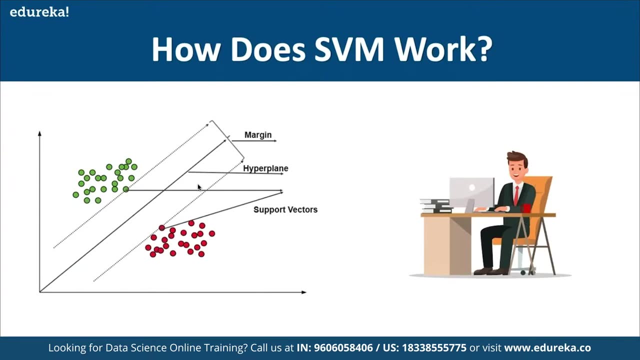 there are different ways of or even on dealing with inseparable or, we can say, non-linear plates as well. so, for example, in some cases hyperplanes cannot be very efficient and in those cases the support vector machine uses a kernel tick from a kernel trick to transform the input into a higher 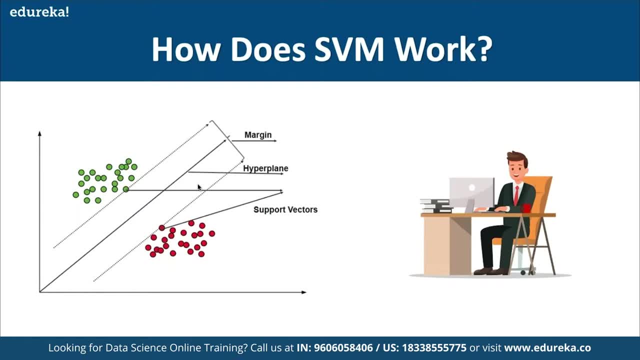 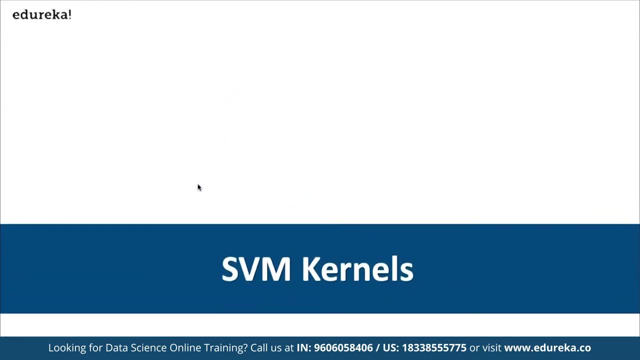 space and with this it becomes easier to segregate the pointers. so now let's talk about the svm kernels. so basically, svm kernel adds more dimension to a lower dimensional space to make it easier to segregate the data. it converts the inseparable problem to separable problems by 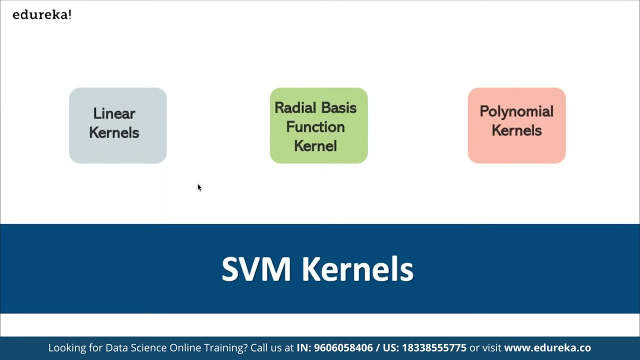 adding more dimensions using the kernel trick and a support vector machine is implemented in practice by a kernel and the kernel trick helps to make more accurate classifier. so we can take a look at different kernels in a support vector machine, like we have linear, we have radial base and then we have polynomial kernels as well as well. let's 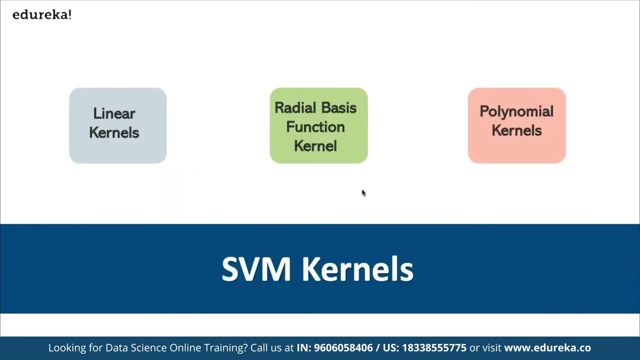 talk about the linear kernels. so a linear kernel can be used to as a normal dot product between any two given observations. so the product between the two vectors is the sum of multiplication of a vector, which is the sum of the following vectors, as shown in the video. 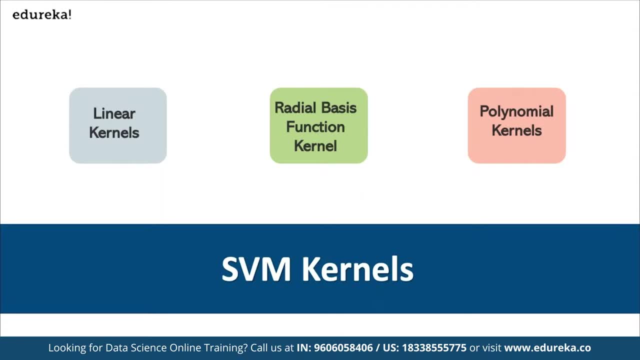 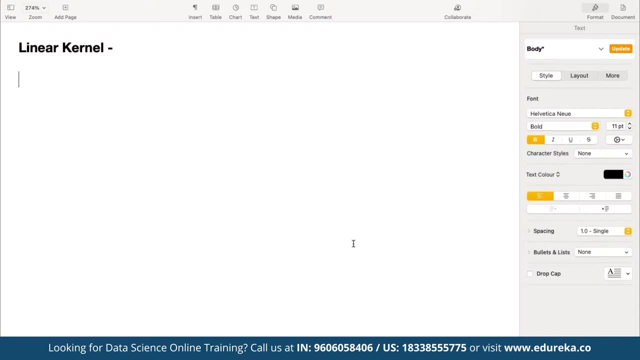 pair input values. so we can understand this. so, if we talk about the linear kernel, so basically, as we as we discussed, linear color can be used as normal dot product. between 82 given observations, for example, here we can find this one as opposed to zero and it can be added to some of, let's suppose, 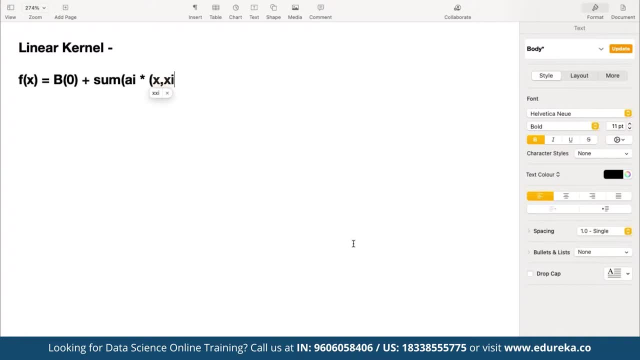 multiplied by X, X, I, alright, so it has been discussed again here. it is going to be the product between two vectors and the sum of multiplication of each pair of input values as a part of simple linear kernel equation. and then we have polynomial, so this one is for linear, then we have for polynomial kernel. so 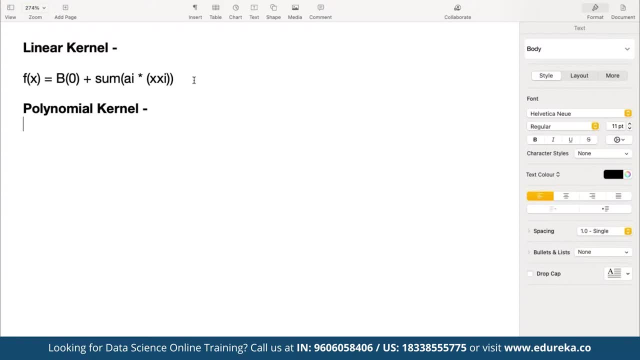 polynomial kernel is for. polynomial kernel is like this. one is for linear, then we have for polynomial kernel. so polynomial kernel is like a is rather generalized form of the linear conta, and again it can distinguish curved or nonlinear input space. so for example, here we can refer this as suppose ask a, and then we can define multiple pointers. I suppose X, 1, X. 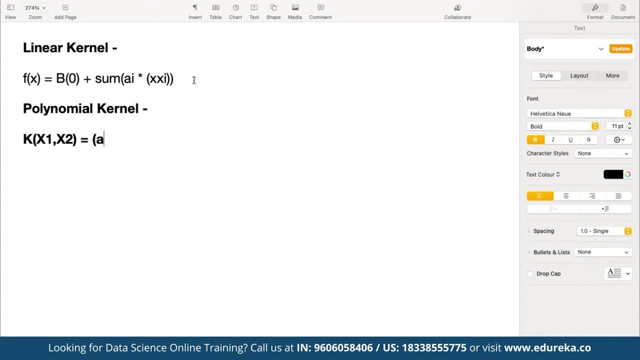 2, and then we can simply add this to a. now here we have device oppose X 1 again, although they could be defined here X 20 and then X 1, for again, in this value for X 2, here two and again the entire one has to be raised to power b itself. so next we after polynomial. 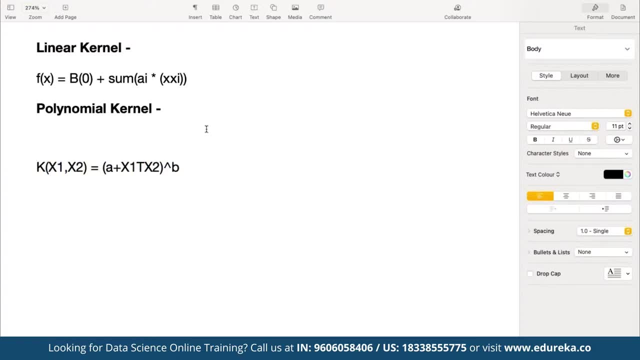 we are going to have, we also have radius space. so here, after polynomial, we have the radial basis function kernel. so in terms of radial basis function kernel, so here the radial basis function kernel is commonly used in the svm classification and it can map the space in infinite dimensions. so basically, if we talk about the actual dimensions here, 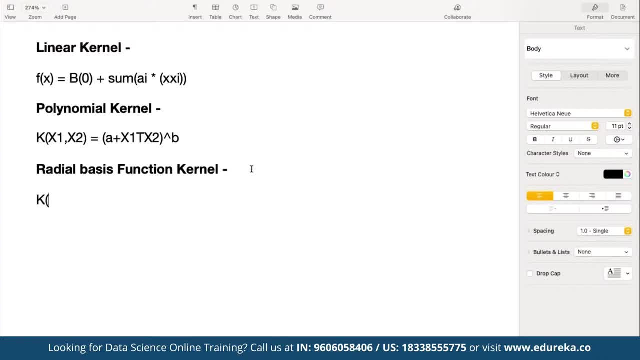 so here we can represent it as suppose the value of k, x 1, and again for x 2, and here we can find the exponent where x period is going to be suppose for minus 4, again the gamma value, and let's say we represent this as y, and then we can define this for: 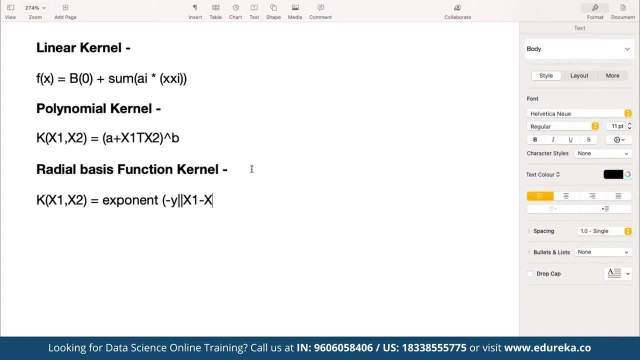 x 1 minus this is going to be x 2, and then it has to be raised to power 2.. so basically, x 1 minus x 2 is simply going to be the euclidean distance between the x 1 and x 2. so we can say x 1 minus x 2. 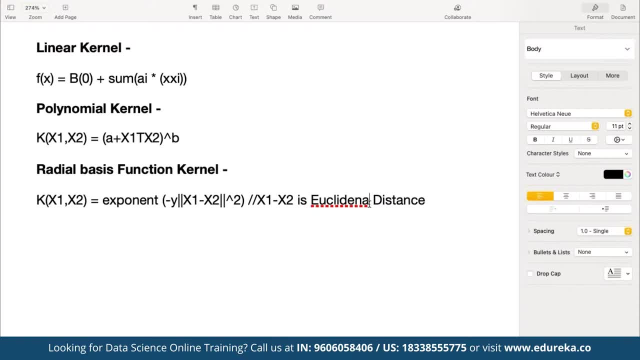 euclidean distance is the euclidean distance between x 1 and x 2, here and where. if we talk about here, if we talk about the current component for b. so here we can say: b is what b is, b is the degree of kernel. in case you don't have, we can, in case you don't have the knowledge of of it yet. 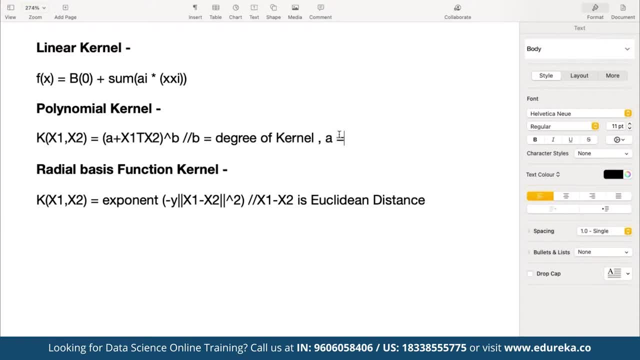 and then a is going to be. or you can say: a is what a is the constant, so b is what a is the constant term that we have. so here we have linear polynomial and then we have radial basis function. so there are multiple use cases. so before we proceed further, 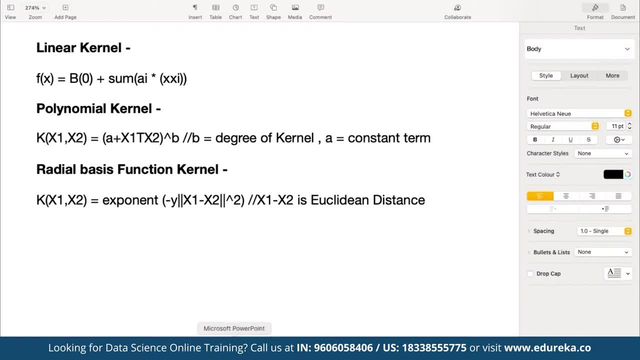 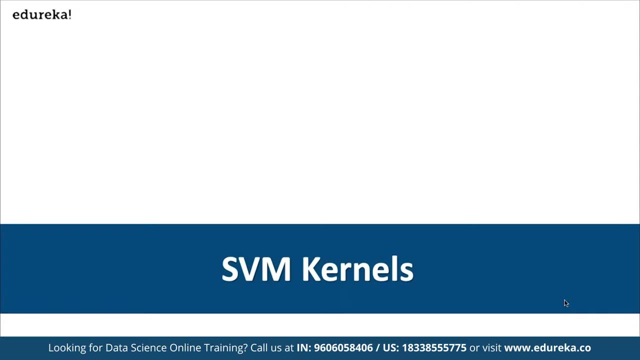 so there are multiple use cases of the serial base conver. i can say component as well. so here we can use it for the phase selection for text and hypertext categorization. here we use it for the classification of images, for bioinformatics, for protein fold and remote homology. 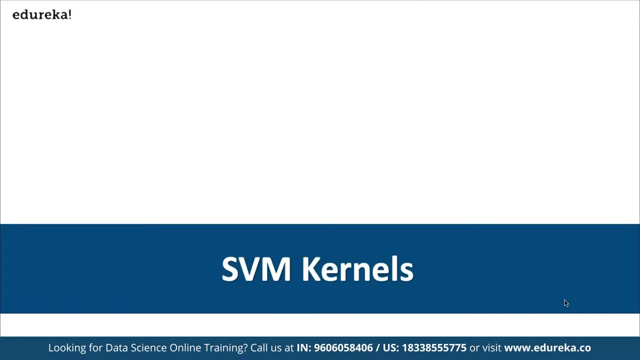 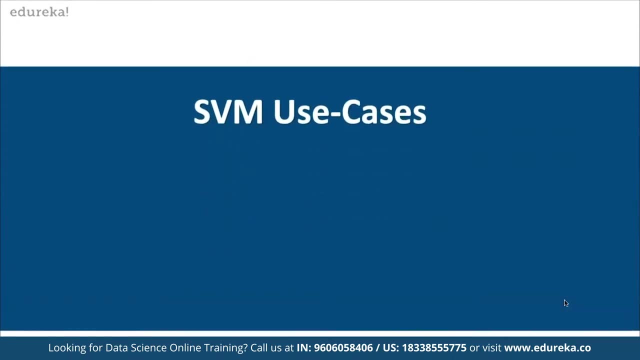 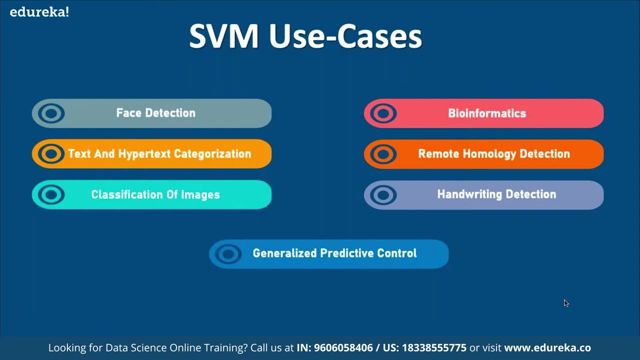 detection as well. we can use it for different use cases and we can also use for again, having a prediction control as well, as we discuss in svm. so there are multiple use cases for face selection, for bioinformatics, for text and hypertext categorization for remote homology. so these 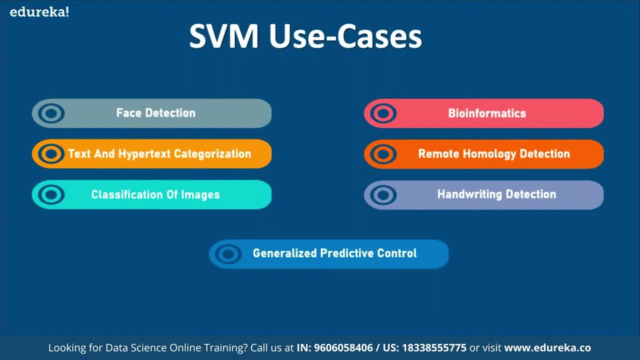 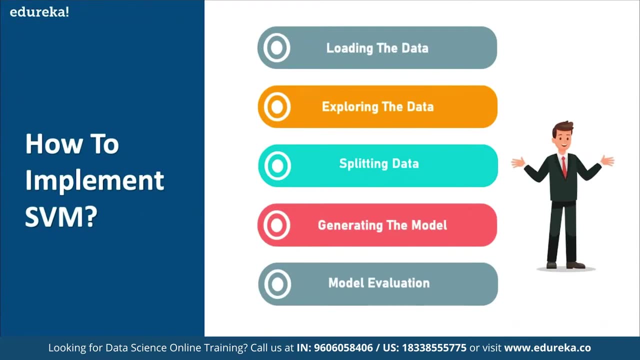 are different use cases are currently available here. so now in terms of how to implement svm. so first of all, we have to load the data, we have to explore the data, we have to split the data, and then we also have to generate the model, and then we have to evaluate the model as well, as we have discussed. again, in case we haven't confused, so 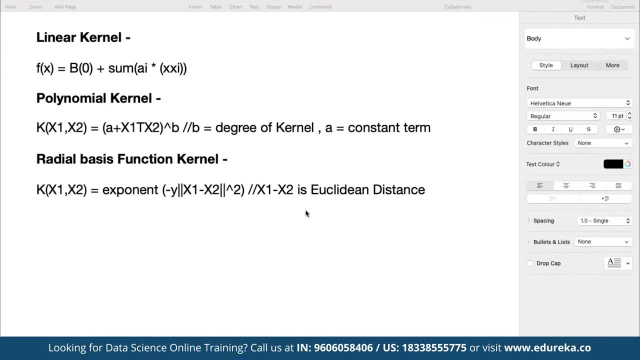 linear is simply going to be the dot product between the any two given observations itself, and here we define two. here the product is going to be between two different vectors, it's simply going to be the sum of multiplication of each pair, and then under polynomial. so basically here we can distinguish curved or non-linear. 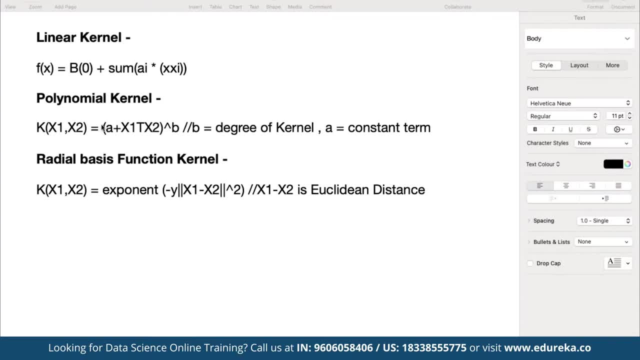 input space where we have defined the k1 as x1, x2 for where a is where a is simply going to be a constant term and b the power to which we have increases. so b is simply going to be the degree of penalty we are going to make use of and then, under radial basis, as we discussed, it is commonly 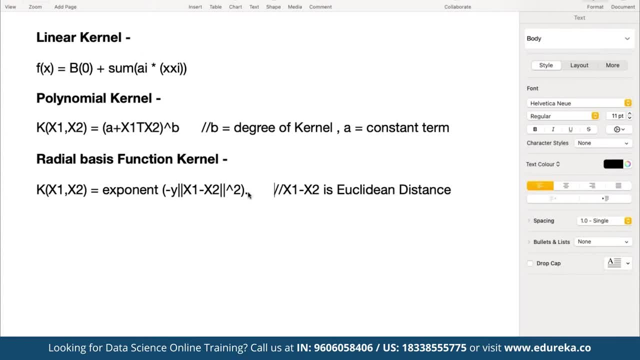 used in classification and can map the space in infinite dimensions as well, where x1 minus x2 is simply going to be the euclidean distance. and we can say this one that we defined here, x1 minus x2 here is simply going to be the euclidean distance here. all right, so 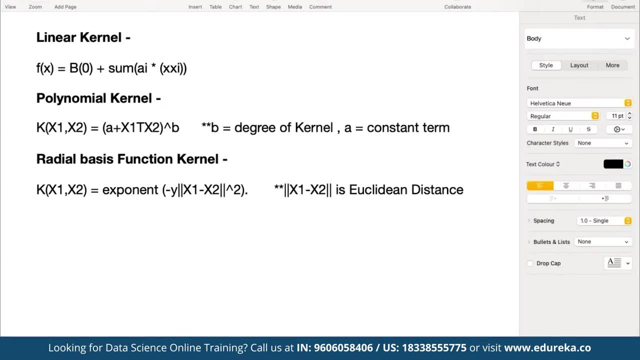 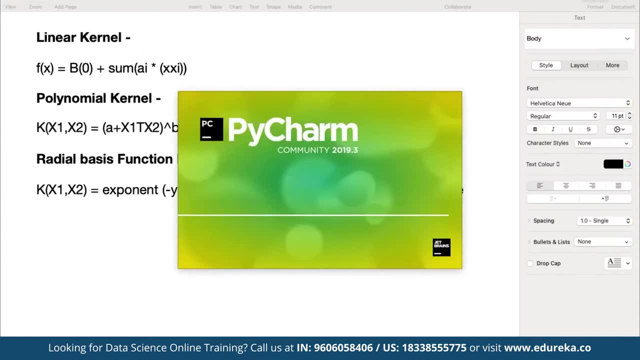 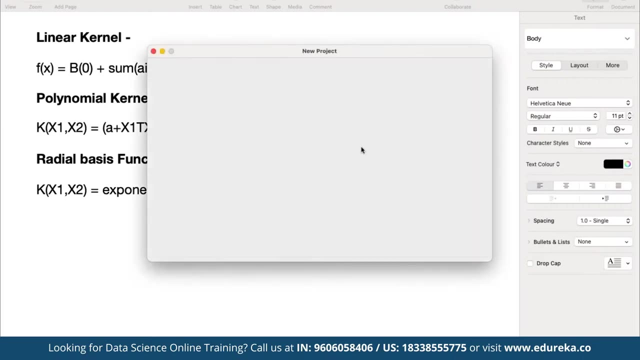 let's do one thing. let's open up pycharm community here so we can start by simply loading the data set and then working on top of it. so we can use any id. we can use any python id to get started. we can use anything. so let's do one thing. let's create a new project. let's say we name it as svm. 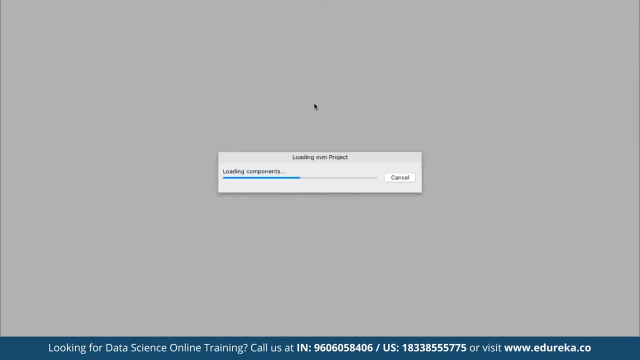 as of now. so in case you don't have the access to svm as of now, so you can go ahead and download the community version. so this is going to give you the access to pycharm, or we can use any other id as well, if required. all right, so here, once we end the project. 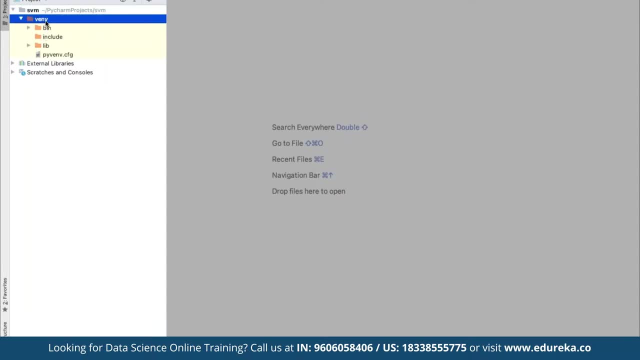 here we can simply go ahead and create a new file altogether, so let's name it as our demo file. so first of all, we are going to work from the skln library, so here we can use from skln. we are going to import the data set, so they they are some sample data set available under 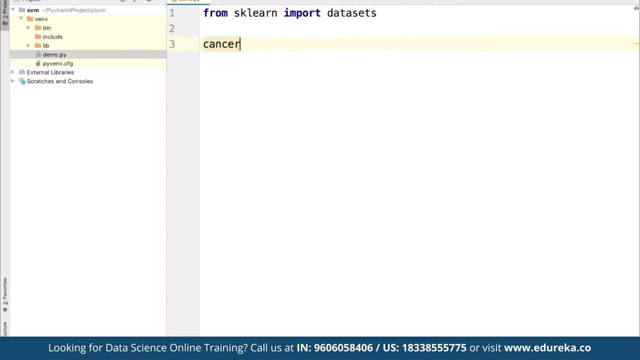 skln library itself. so here we can define the cancer data set already available under skln and here we can use data set, start load and then we are simply going to load support for breast cancer. we can load this current data set already available. and now, if we want to simply print the current data set that we is, that we have currently imported, 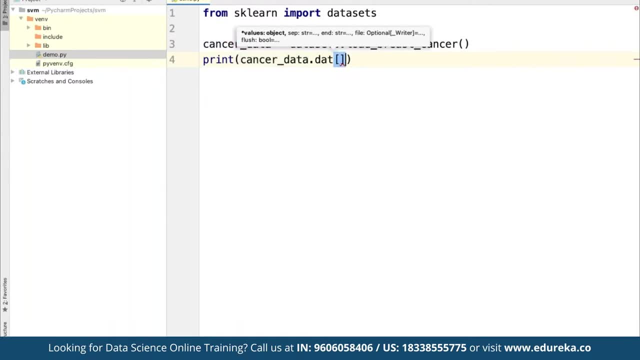 so here we can find cancer data, dot data, and again we only want to print the five first rows available in that. so here we can define these statements here. so we have. we are going to use the sample data set currently available and whenever we are going to work on any project. 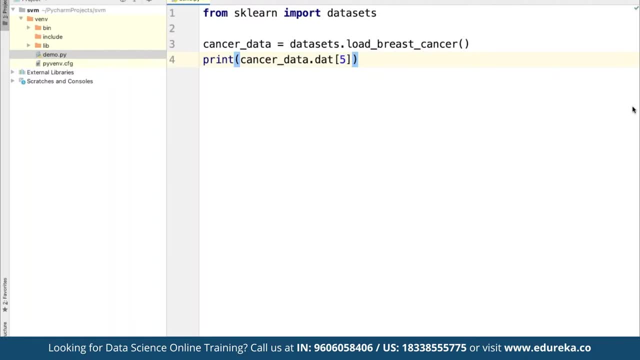 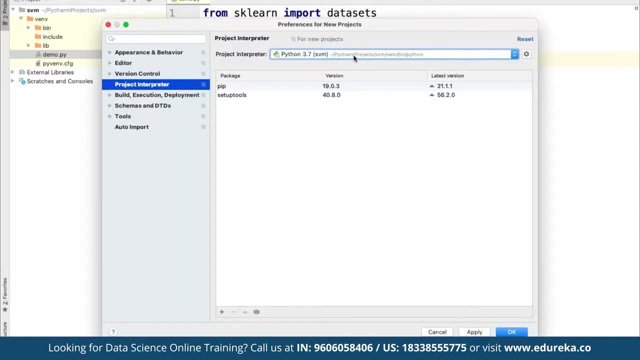 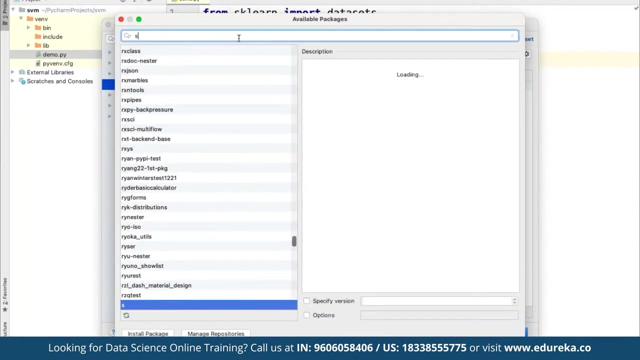 in case they are now, in case the data set is not available, then we can go ahead and simply install more libraries by simply choosing the current data set and then here we can go ahead and click on add and from here we can search for any library. that is that we may that may be missing. 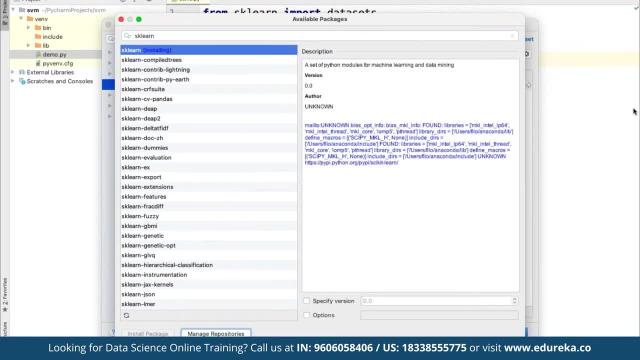 for example, here we are going to work on skln, so we have to make sure that we do import skln, because without skln library we will not be able to work on the svm here. so here we are simply going to work on the sample data set. all right, so as you can see, now skln has been installed. so again, 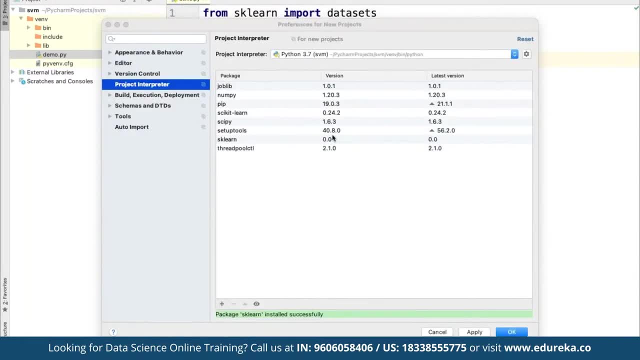 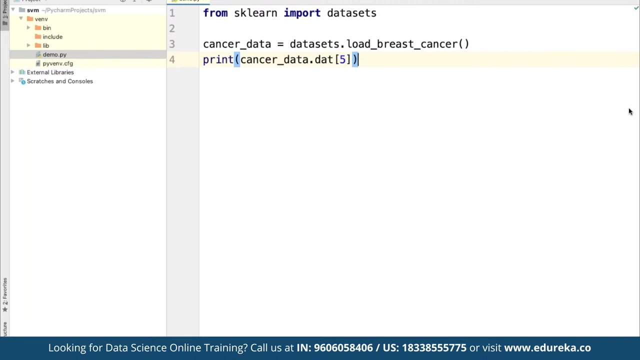 this is a package that we're going to work with, so here we can close it. if we want to work on the other components, we can search for any library and then we can have it installed. all right, so now we can click on apply and then once we talk- because if we don't have the library installed, 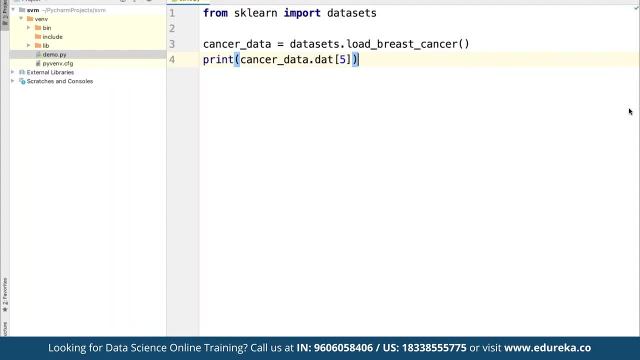 and then, if we try to run the sub, it will simply go to throw us an error and, as you can see, currently this is going to update the package and then from there, it is simply going to load the breast cancer data set that we have already imported. so we can just tell it to run the sub. 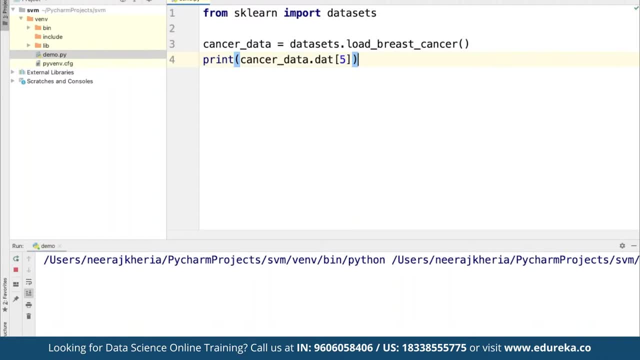 data set which is available as an inbuilt sample in SQL. so it is simply going to get connected to the server and then from there it is going to be going to pull the load, the breast cancer leader said, and then it is simply go to print the first five rows from that data set. so it may take a while, depending. 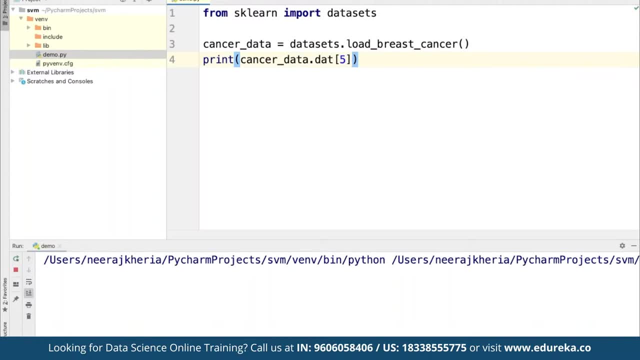 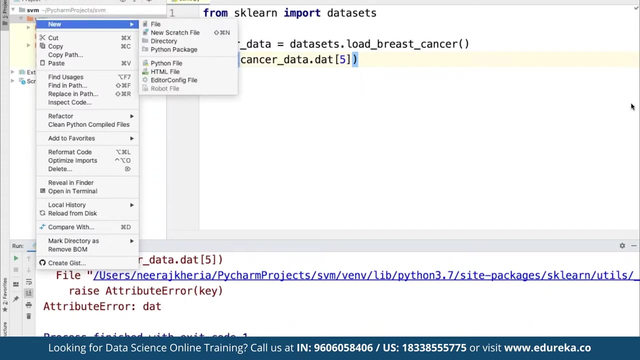 upon how which data set we have imported. so before we perform any calculation, let me just show you how started this looks like. again, in the meantime, this is getting pull here, so we can simply go ahead and create a new file. it has been timed out because of memory error. 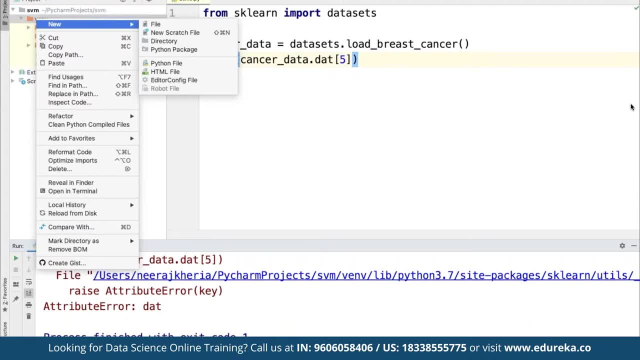 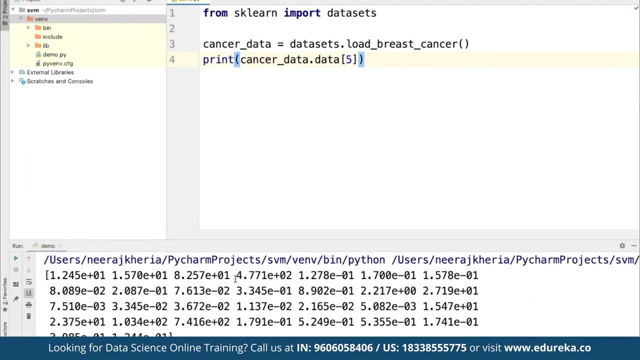 okay, we defined, we misspelled data. it has to be data itself then. only it is simply going to fetch data from there. so, as you can see here, now we have the first five rows in terms of this breast cancer data, which has been pulled automatically from sklan, as you can see here. 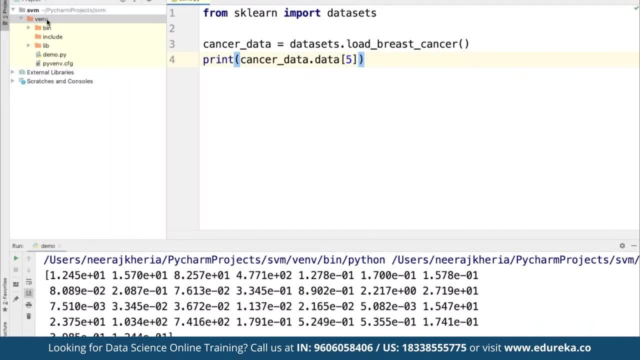 right. so now we are going to here. we have defined the data set right. so now, if we are going to simply split the data, right? so we are simply going to divide the data into training said, and the test set to get accurate results, and after this we will split the data using the train test split function. so here we are. 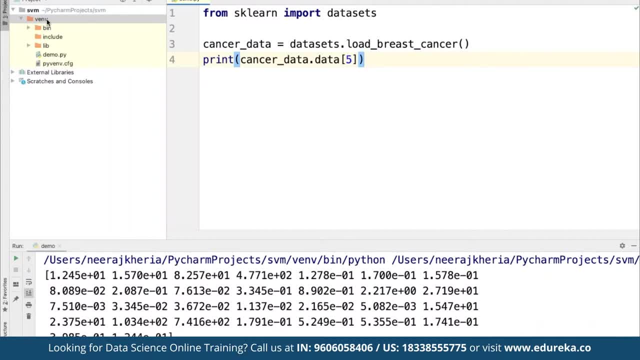 going to need three parameters, like in the example that we have that we are going to see. so from here we are going to load the current data set. so, for example, here now, just to avoid confusion for yours, so we can create a new file. let's say we define sense as: 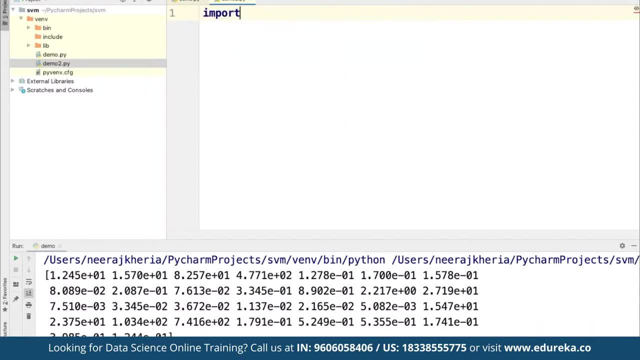 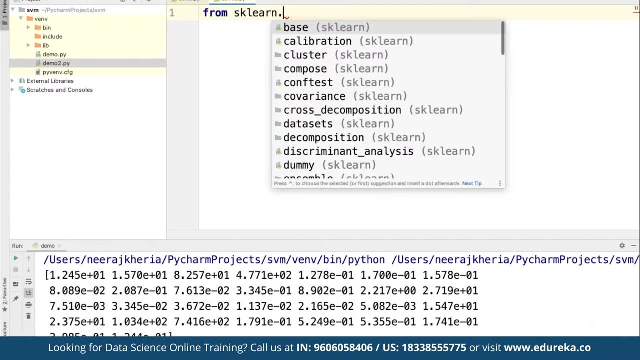 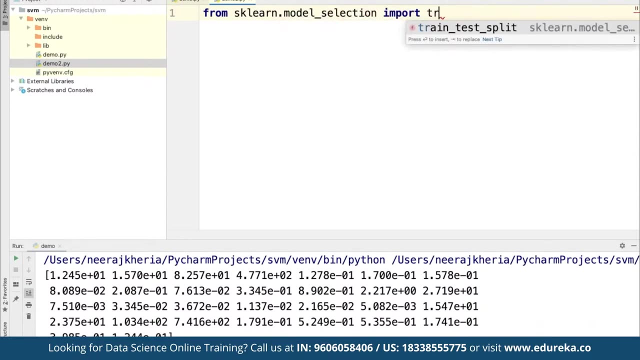 suppose number two. so here we can define from sklearn. so first of all we define from sklearn library, from sklearn dot model, and here we can define model selection. so here we are going to import train test split, as we discussed, we are going to split it and then we can define from. 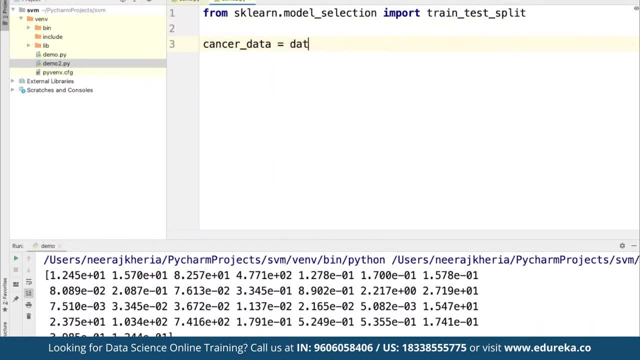 cancer data that we are going to import. so here we are going to find data set, dot load, rest cancer, which is already available, and then we are simply going to define the models in terms of: suppose, here we define x train, and then we can find x split. 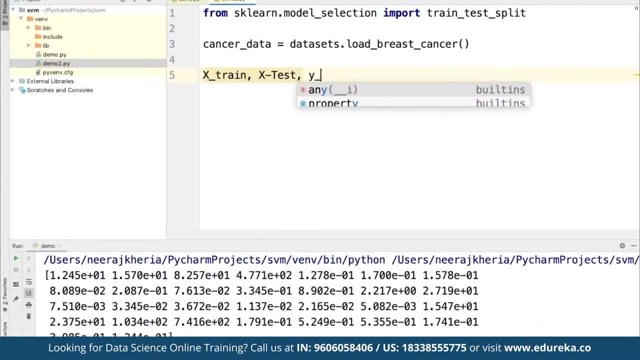 uh, we can define for x test, and then we can define same thing for y train, for y test, x train, x test, y train, y test. so here we are going to define this from the same train test split that we are going to import, and then here we are going to divide them under. 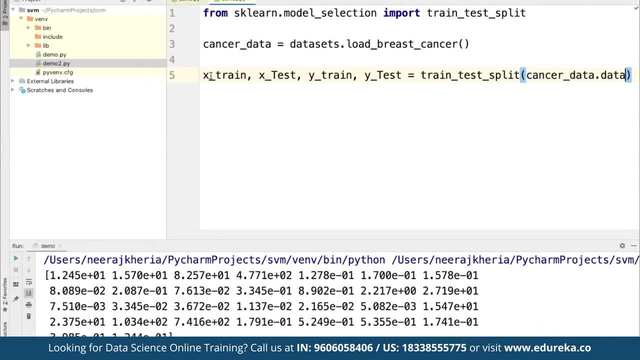 from the cancer data and the data which has been imported here, and then we are going to define this for cancer data target. so say, here we can define this for cancer data dot target and then we can define the test size. here we can define the test size. suppose we want to keep the test size, suppose, as four. 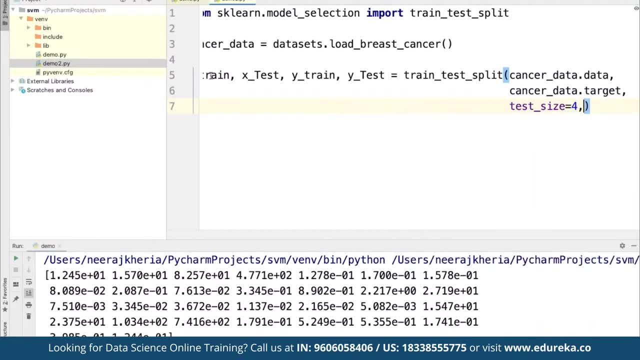 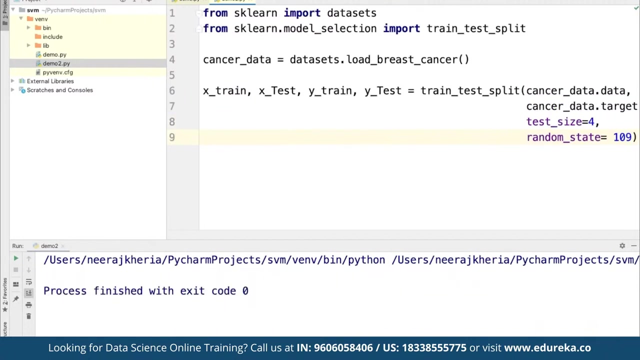 this test has s4, and then we can define random state. we can define random state and suppose that's the Ferguson in fantasy. i understand that maneira horsepower. so so we are going to generate data set and then we can, because, for example, here we can put radiop battle and here we are going to generate the model as well. so what we can do is so, now here we are going to change, we can. 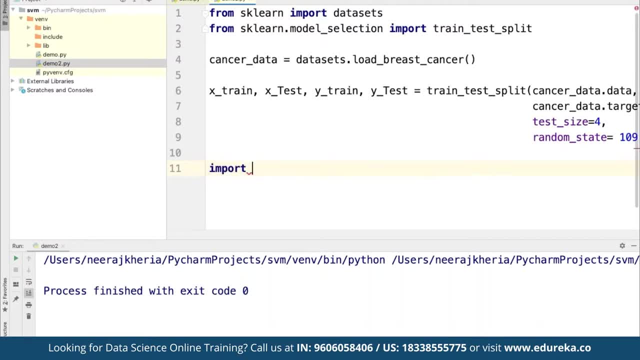 generate the model, and for that we can import analog. for example, here we four on another honeyton, and then we can see: now here we can, and the data setவ import, let's say a scalar, and here from escalant we are going to import the svm. so here we are. 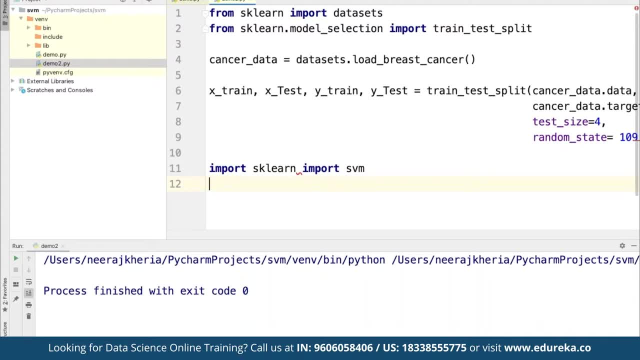 going to create the library, so here we could create a classifier here. so first of all we're going to find classifier as opposed svm, dot, svc, and here we can find the kernel. here we can find the kernel as opposed linear, whatever we want to use, we can define that, and then we are going to 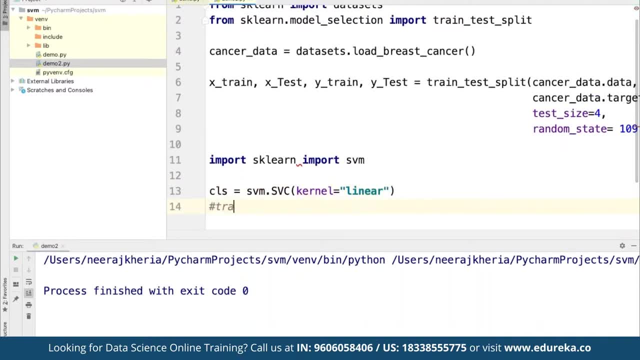 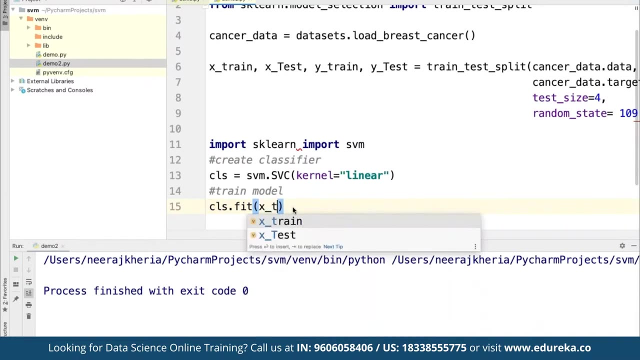 train the model. so you can see, we are simply going to now train model. so here we have create classifier and now we are going to train the model. so for training one, we can define class dot, fit, and then we can define this value as x train that we have already imported, and then we can. 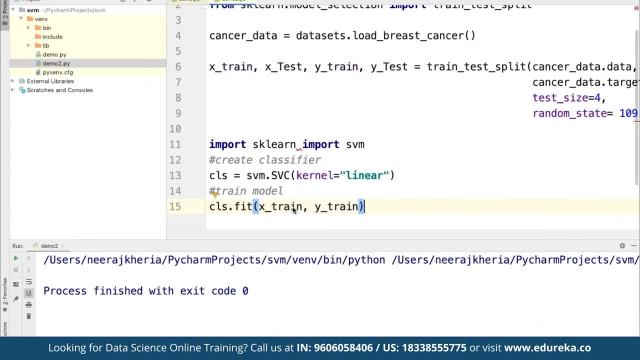 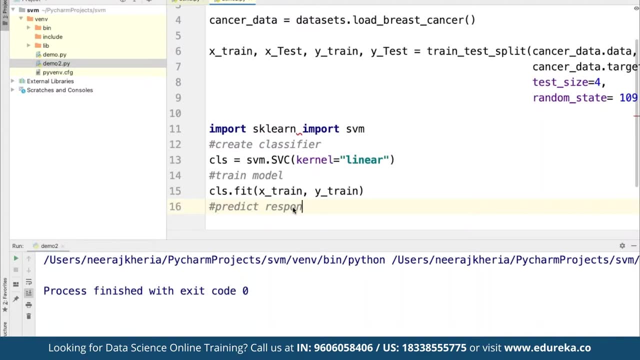 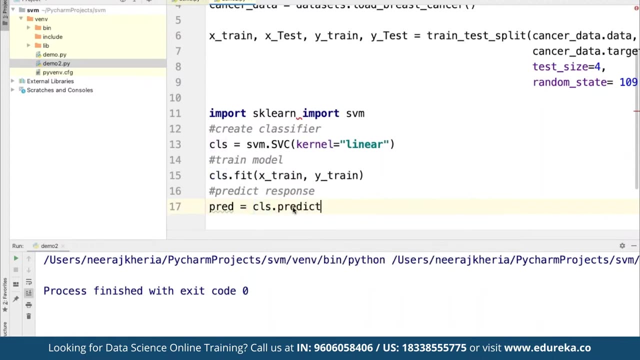 define for y train that have, we have already performed the split on and then simply, we are going to have a prediction done. so here we can define prediction response and for getting the response we can define prediction as class dot, predict. and for this we are going to make use of x test that we have already defined. we define for x train. 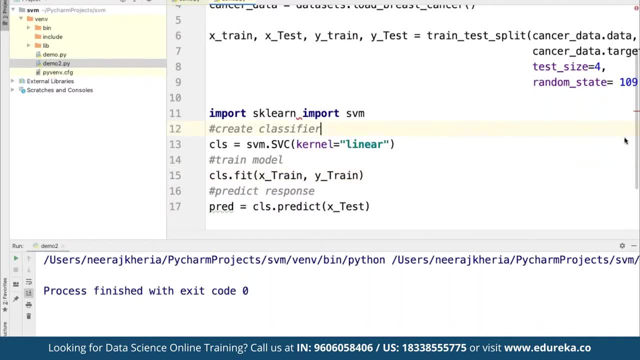 and for y train and then for prediction. we are simply going to do that on the text on the x underscore test that we already have defined. that depends upon type of data that we have. so that totally depends upon the type of data we are going to simply import and let's move this import from the end up here. 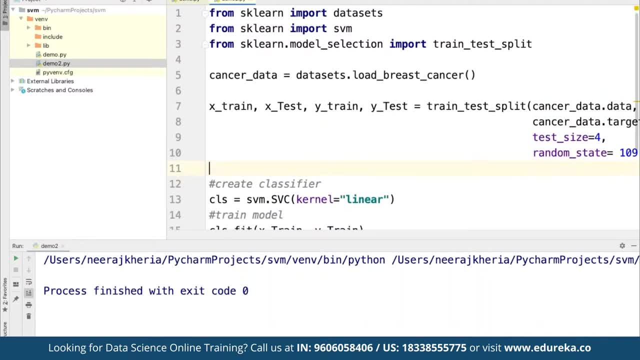 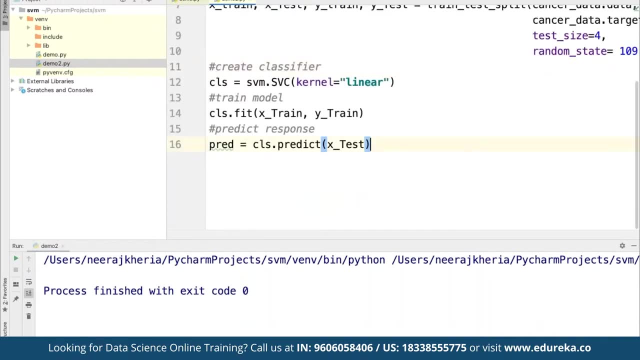 so you have to define this in the top section from sql. we are simply going to import the svm. if we had to find, all right, and now we have to find the classifier. now we are going to evaluate the model and for evaluating the model, we can simply go ahead and define. 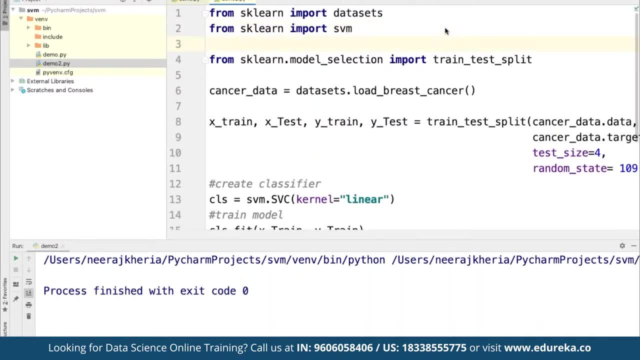 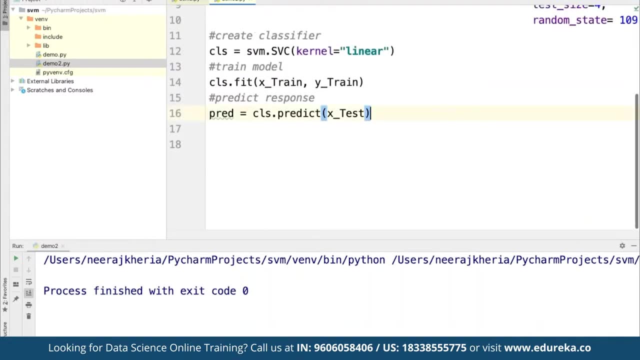 so here from s killer we can also import other components as well. from sql we are also going to import metrics. so here we are also going to import metric, and by using macro accuracy, metric for getting the accuracy we can find, for getting the accuracy we are going to define, we are simply 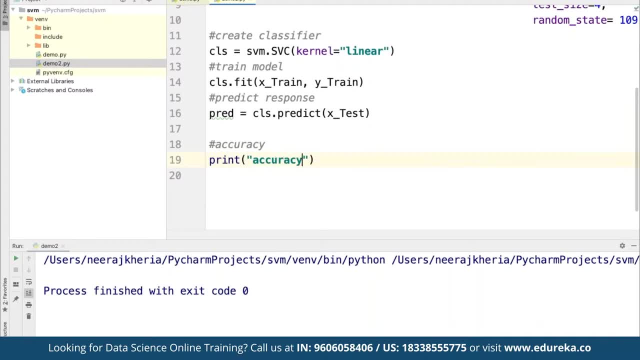 going to print the accuracy of the prediction here and for accuracy, we are simply going to define metrics, which is again available under the matrix that we here we have accuracy score and then from here we are simply going to find wire test and we are going to find this before why prediction as well, that we have defined. 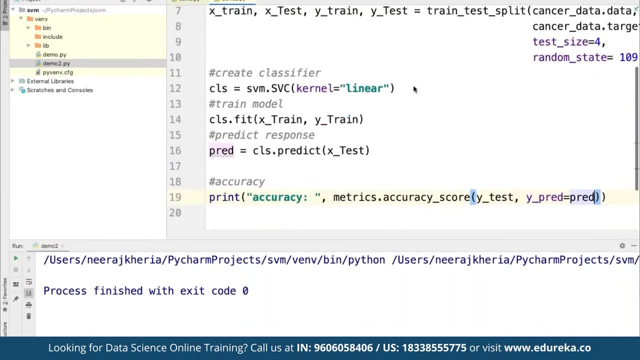 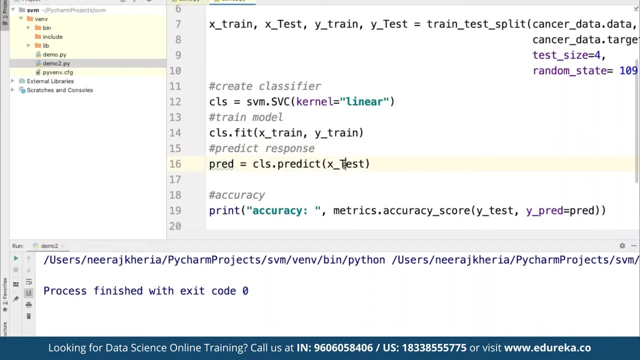 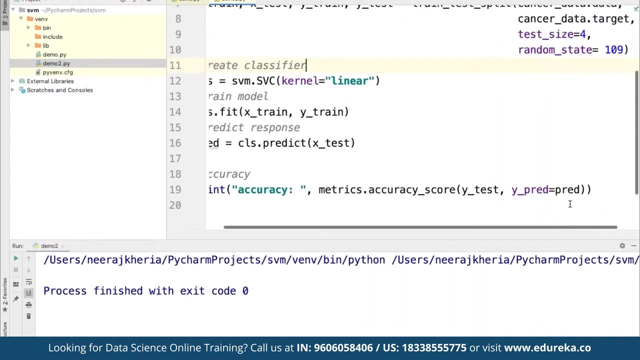 so i think we have used y test, we have used upper case for before, we have used let's do one thing, let's use small case for everything. just to avoid confusion. let's find this test, train and test again. so you have your y test and then you depend here. we define it for production and then for 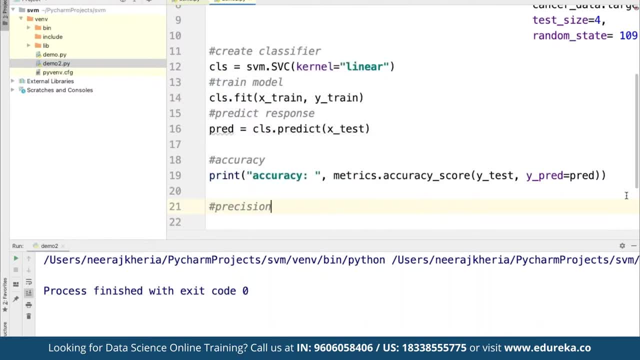 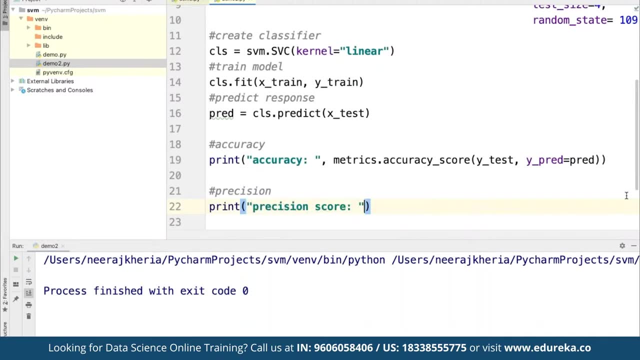 finding the precision score. we are going to find the precision score. we are going to find the precision score for finding precision. we can simply print another statement as precision score, and in here we can again make use of metrics, and for metrics we can define the precision score itself. so here we can define precision underscore score and here 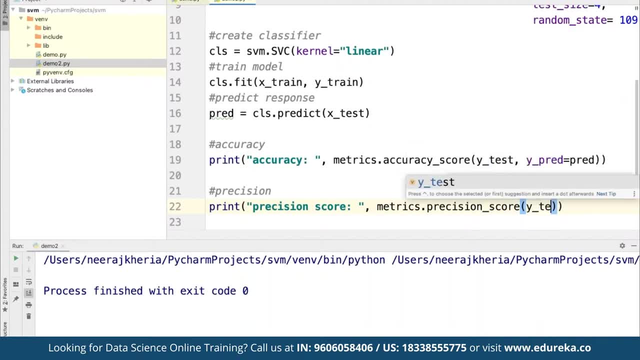 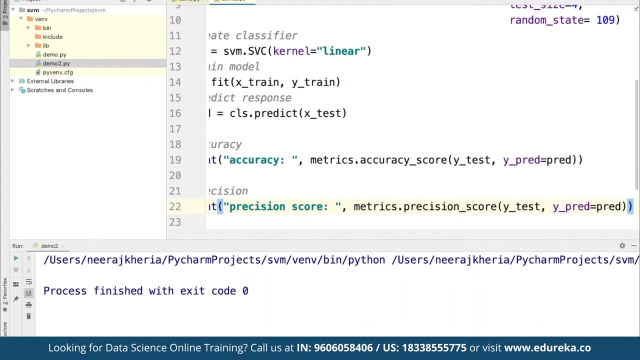 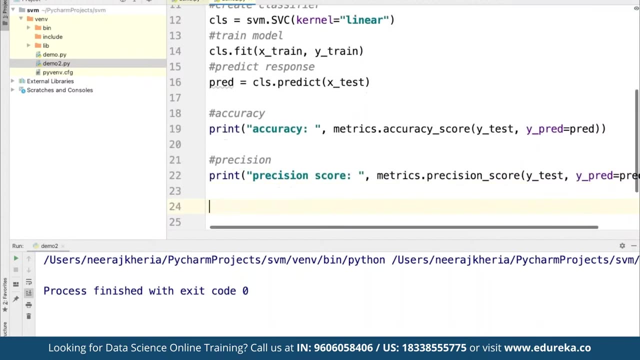 for precision score, we are going to make use of y test, and then we are going to make use of y test, then we are going to make use of y prediction, all right. and then at the end, if you are simply going to recall the score and we are simply going to report, so here we can define for recall.